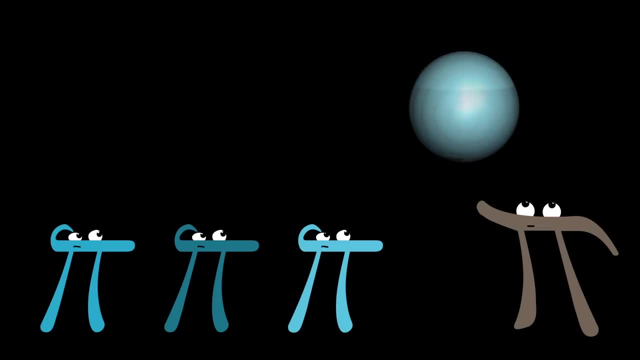 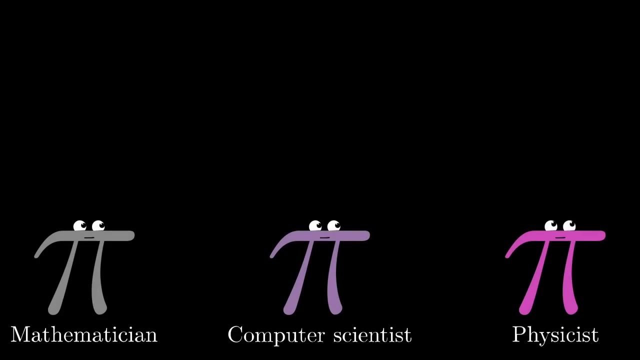 forth. I mean it is reasonable to imagine that there are problems out there that would have clever and illuminating solutions if only we knew how to conceptualize, say, lists of ten numbers as individual points in some space. For mathematicians or computer scientists or physicists, problems that are framed in 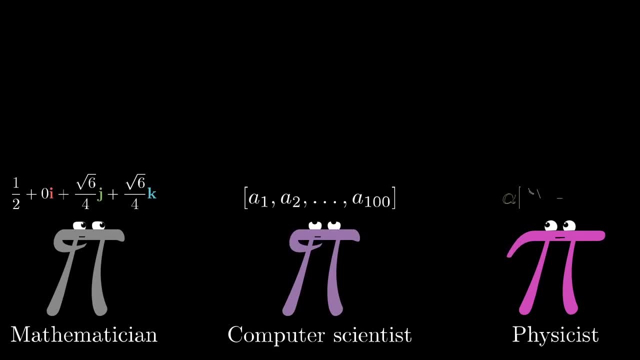 terms of lists of numbers. lists of more than three numbers are a regular part of the job, And the standard approach to actually doing math in higher dimensions is to use two and three dimensions for analogy, but to fundamentally reason about things just analytically somewhat. 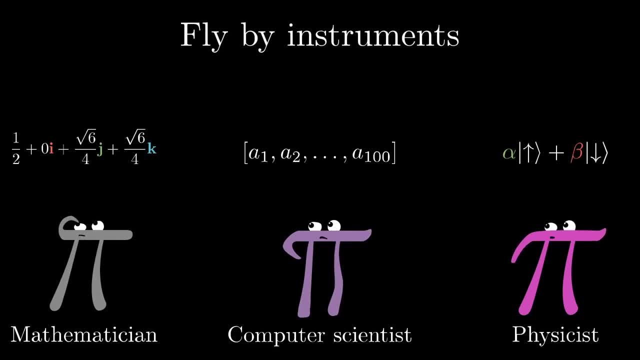 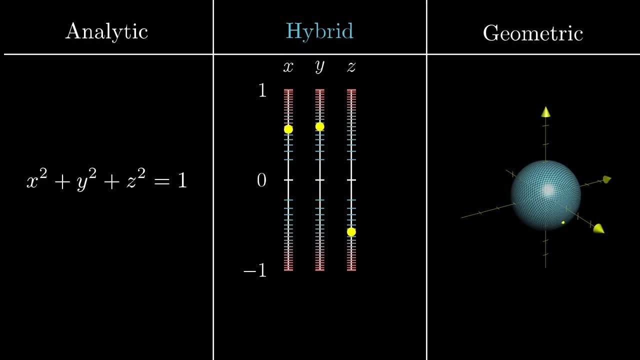 analogous to a pilot relying primarily on instruments and not sight while flying through the clouds. Now, what I want to offer here is a hybrid between the purely geometric and the purely analytic views, a method for making the analytic reasoning a little more visual, in a way that 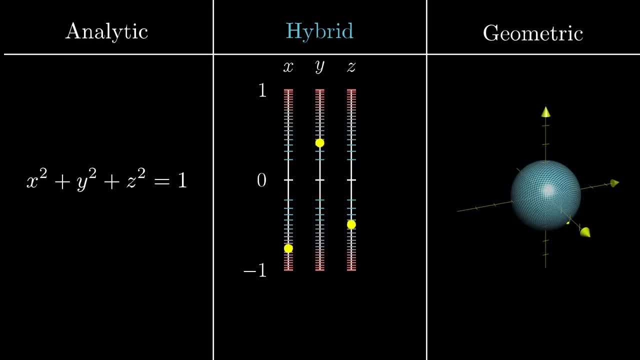 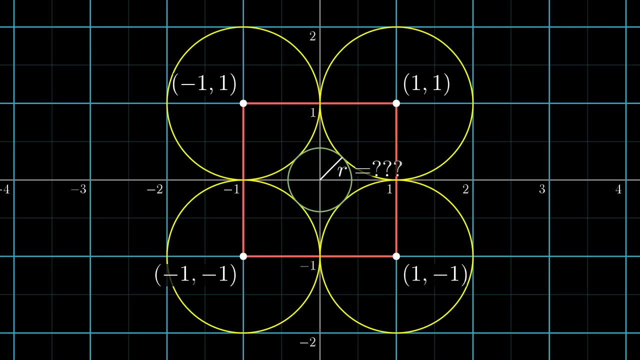 generalizes to arbitrarily high dimensions And to drive home the value of a tactic like this, I want to share with you a very famous example where analogies with two and three dimensions cannot help because of something extremely counterintuitive that only makes sense. So let's look at an analogy with two and three dimensions. Let's look at an analogy with two and three dimensions. Let's look at an analogy with two and three dimensions In a more than three dimension approach. the goal is to bring out this magnetic field. 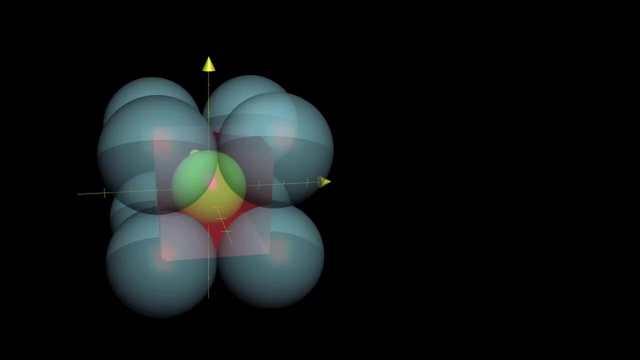 of the electron in the atom. So let's look at an analogy with a four-dimensional sphere that is centered at the origin, and see what happens in higher dimensions. The hope, though, is that what I show you here helps to make this phenomenon more intuitive. 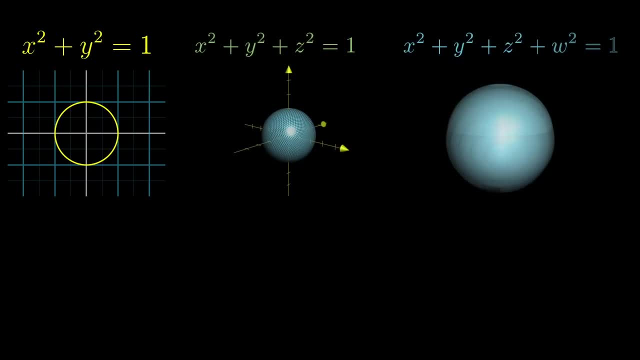 The focus throughout will be on higher dimensional spheres. For example, when we talk about a four-dimensional sphere, say, with radius, one centered at the origin, what that actually is is the set of all quadruplets of numbers, where the sum of the squares of these numbers is one. 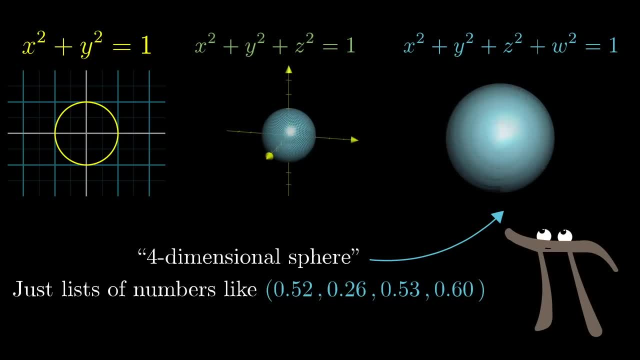 dimensional slices of a 4D sphere projected back into three dimensions. But it's confusing and even if you do wrap your head around it, it just pushes the question back to how you would think about a 5, or a 6, or a 7 dimensional sphere. 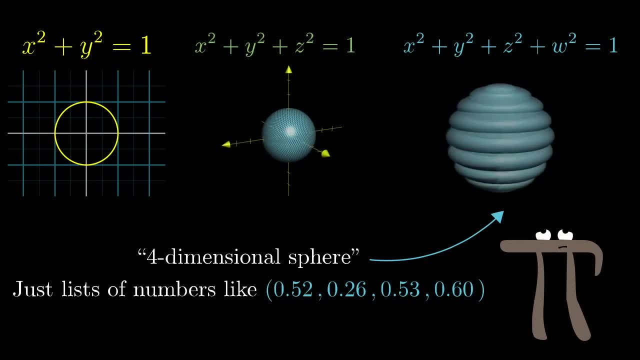 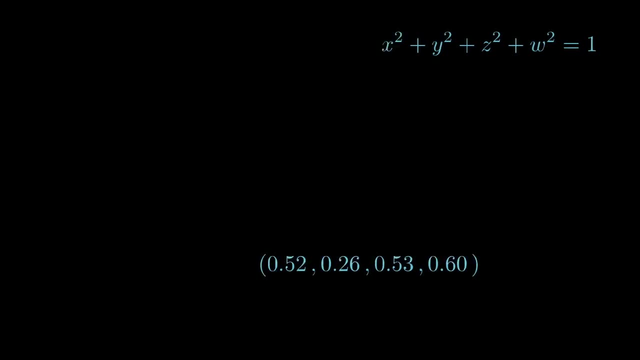 And, more importantly, squinting your eyes to understand a projection like this is not very reflective of what doing math with a 4D sphere actually entails. Instead, the basic idea here will be to get very literal about it and to think about. 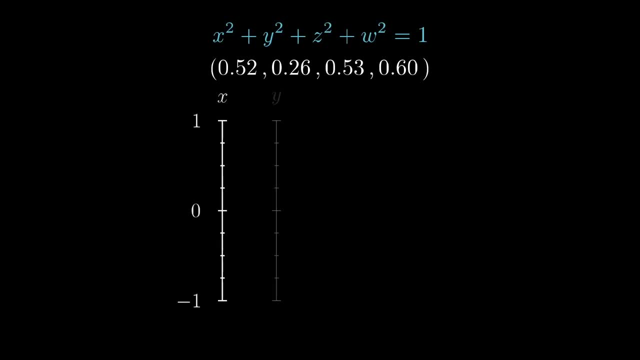 four separate numbers. I like to picture four vertical number lines with sliders to represent each number. Each configuration of these sliders is a point in 4D space, a quadruplet of numbers, And what it means to be on a 4D sphere centered at the origin is that the sum of the squares. 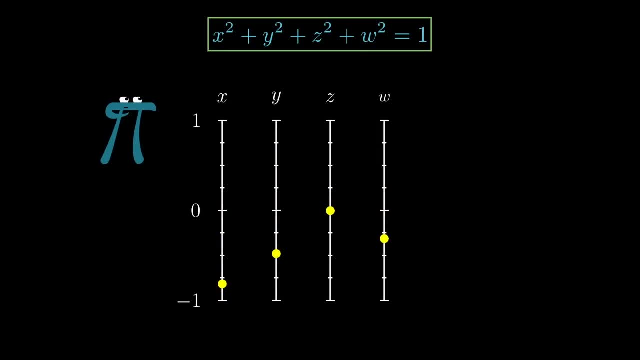 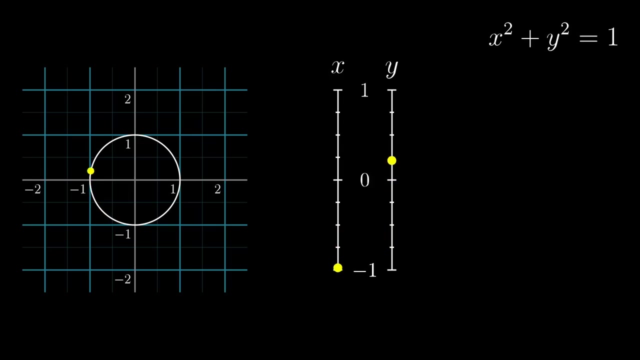 of these four values is: 1. Our goal To understand which movements of these sliders correspond to movements on the sphere. To do that, it helps if we knock things down to two dimensions, where we can actually see the circle. So ask yourself what's a nice way to think about this relation that x squared plus y. 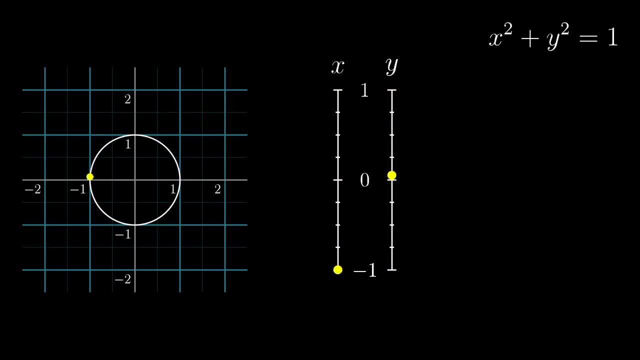 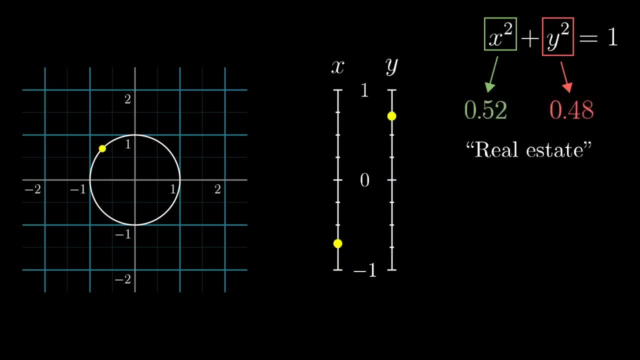 And that they have a total of 1.. And that they have a total of 1.. And that they have a total of 1.. So moving around on the circle corresponds to a constant exchange between real estate and the variables. I choose this term because it lets us make an analogy: that real estate is cheap near 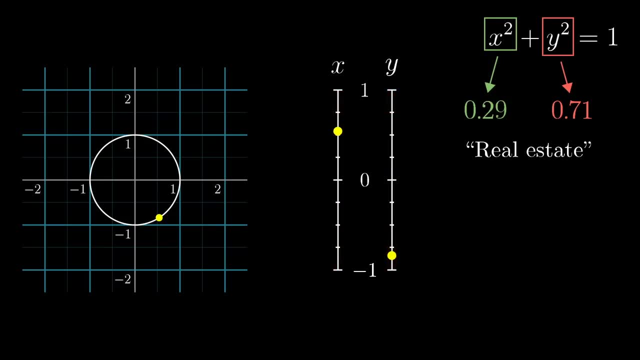 zero and more expensive away from zero. To see this, consider starting off in a position where x equals 1 and y is zero, Meaning x has all of the real estate to itself which in our usual geometric picture would, which means we're on the rightmost point of the circle. 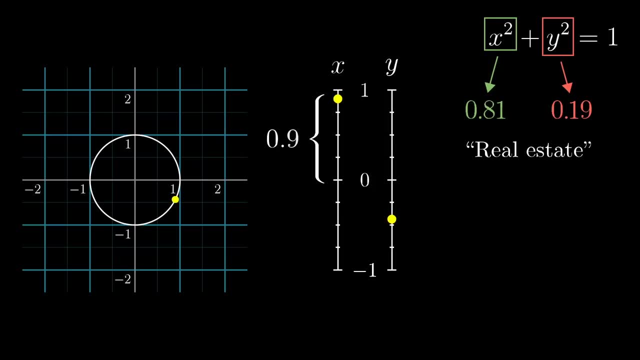 If you move x down just a bit to 0.9,, the value of x squared changes to 0.81, so it has in effect given up 0.19 units of real estate. But for y squared to increase by that same amount, y has to move an entire 0.44 units. 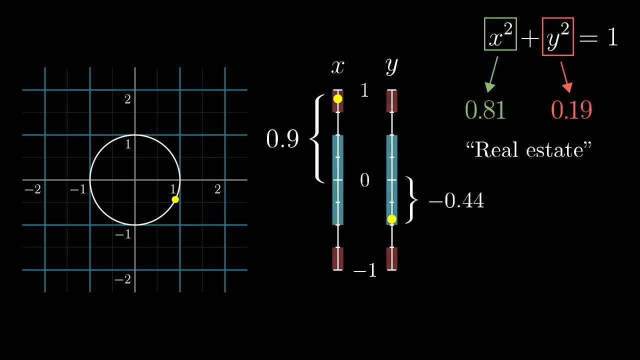 away from 0, more than 4 times the amount that x moved. In other words, x changed a little to give up expensive real estate so that y could move a lot and gain the same value of cheap real estate. In terms of the usual circle drawing, this corresponds to the steep slope near the right. 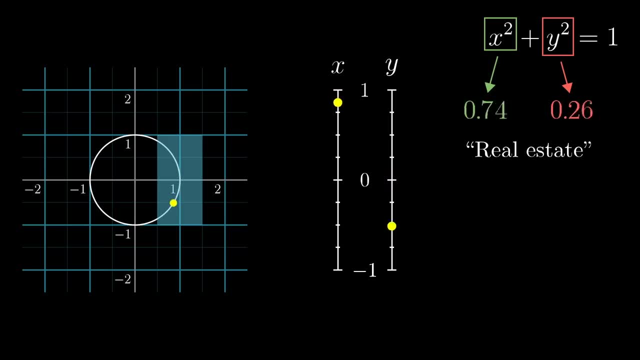 side, A small nudge in x allows for a very big change to y Moving forward. let's add some tick marks to these lines to indicate what 0.05 units of real estate looks like at each point. That is, how much would x have to change so that the value of x squared would be 0.05? 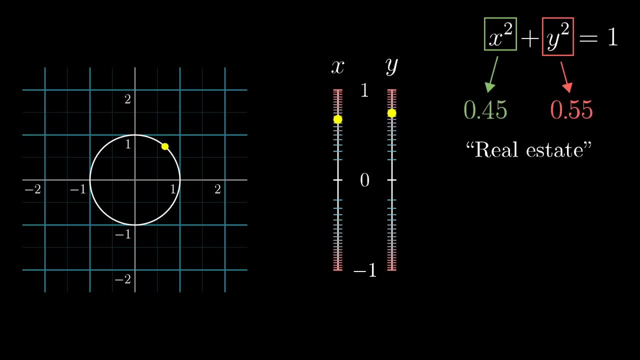 units. As you walk around the circle, the tradeoff in value between x squared and y squared gives this piston-looking dance motion, where the sliders are moving more slowly away from 0, because real estate is more expensive in those regions. There are just more tick marks to cover per unit distance. 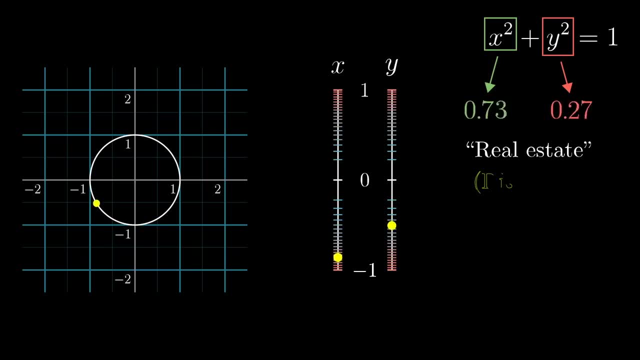 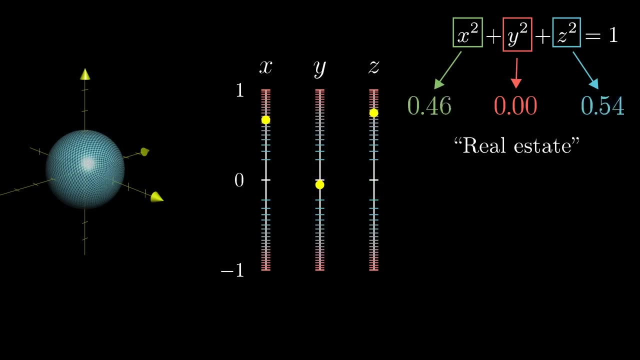 Also a nice side effect of the term real estate is that it aligns naturally with the fact that it comes in units of distance squared. So The square root of the total real estate among all coordinates gives us the distance from the origin For a unit sphere in three dimensions, the set of all triplets xyz, where the sum of their 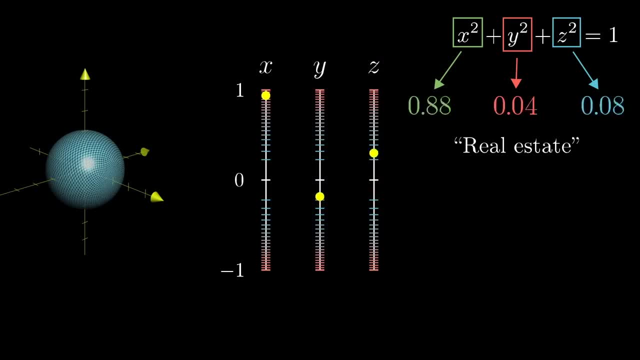 squares is 1,, all we have to do is add a third slider for z, But these three sliders still only have the 1 unit of real estate to share between them. To get a feel for this, imagine holding x in place at 0.5,, where it occupies 0.25 units. 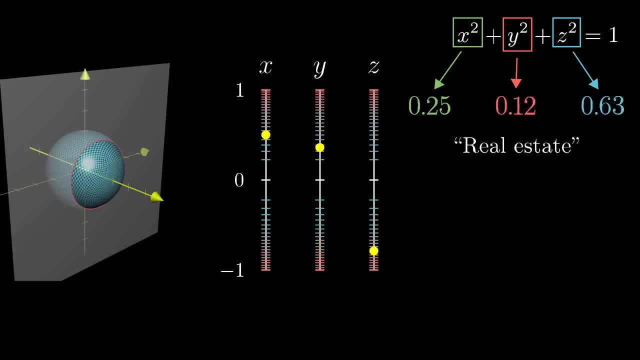 of real estate. Okay, What this means is that y and z can move around in the same piston-dense motion we saw before, as they trade off the remaining 0.75 units of real estate. In terms of our typical way of visualizing a sphere, this corresponds to slicing the. 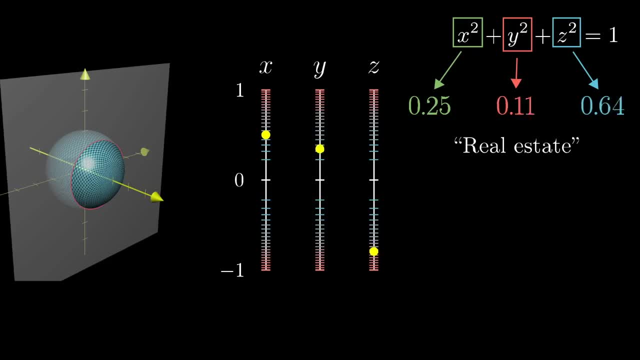 sphere along the plane where x is 0.5 and looking at the circle formed by all the choices for y and z on that sphere, As you increase the value of x, the amount of real estate left over for y and z is smaller. 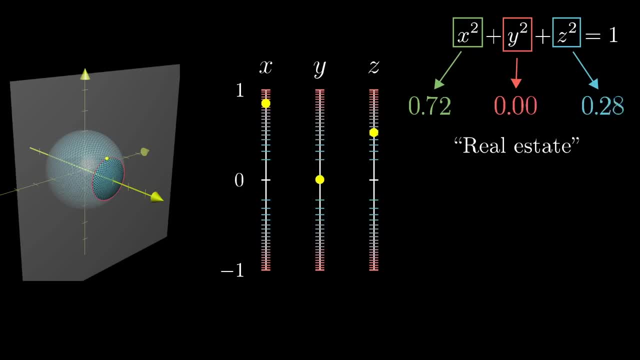 and this more constrained piston-dance is what it feels like for the circular slice to be smaller Eventually. once x reaches the value 1, there's no real estate left over. so you reach this singularity point where y and z are both forced to be 0.. 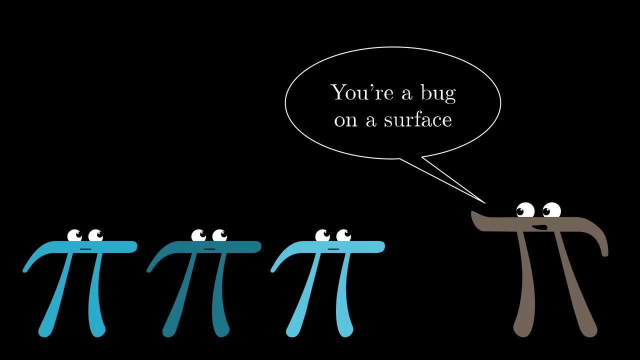 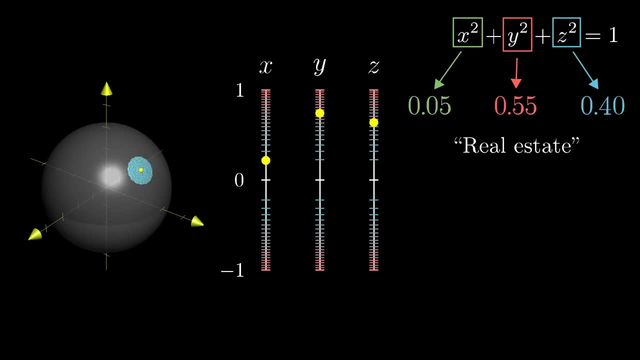 The feeling here is a bit like being a bug on the surface of the sphere. You are unable to see the whole sphere all at once. Instead, you're just stuck. You're just sitting on a single point and you have some sense for what local movements. 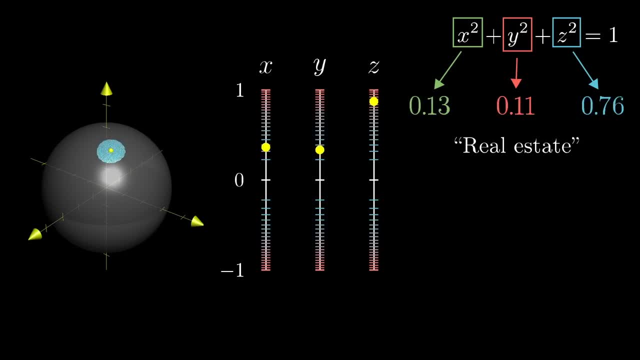 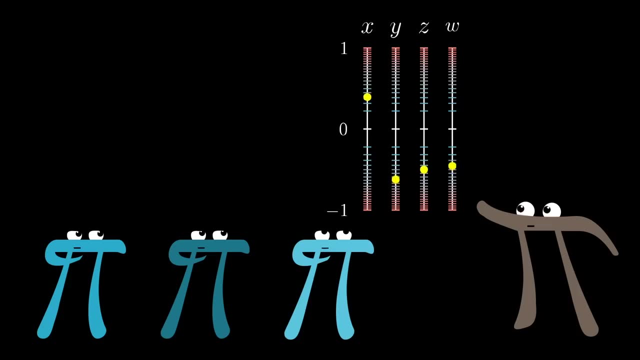 are allowed In 4 dimensions and higher, we lose the crutch of the global view that a spatial visual offers, But the fundamental rules of this real estate exchange remain the same. If you fix one slider in place and watch the other three trade off, this is basically what. 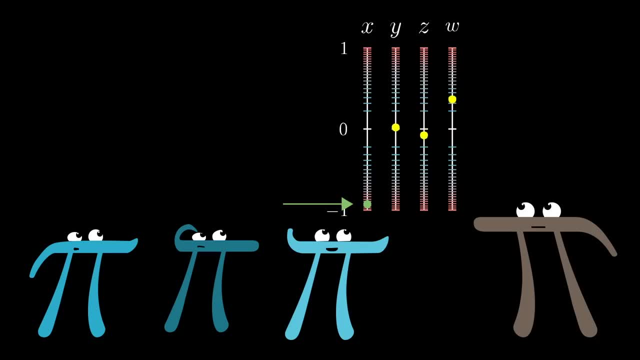 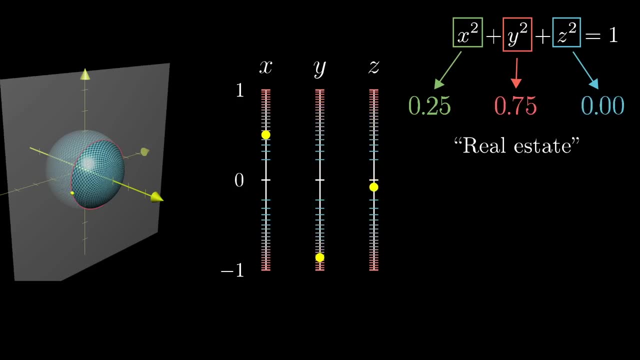 it means to take a slice of the 4D sphere to get a small 3D sphere, in much the same way that fixing one of the sliders for the 3D case gave us a circular slice when the remaining two were free to vary. 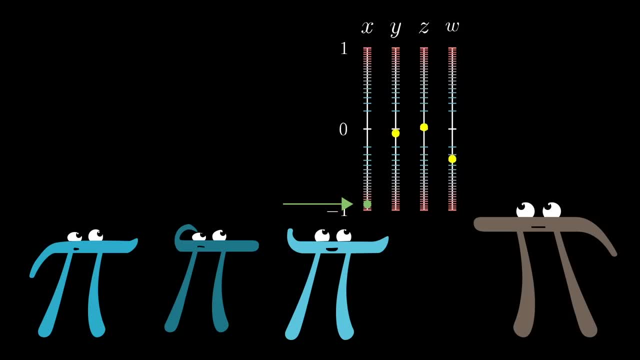 Now, watching these sliders move about and thinking about the real estate exchange is pretty fun, but it runs the risk of being aimless unless we have an actual high-dimensional puzzle to sink our teeth into. So let's set aside the sliders for just a moment and bring in a very classic example. 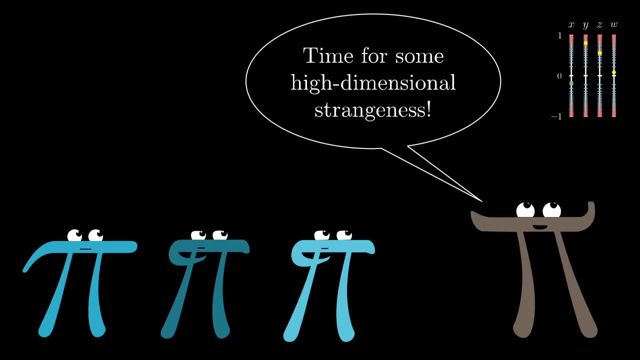 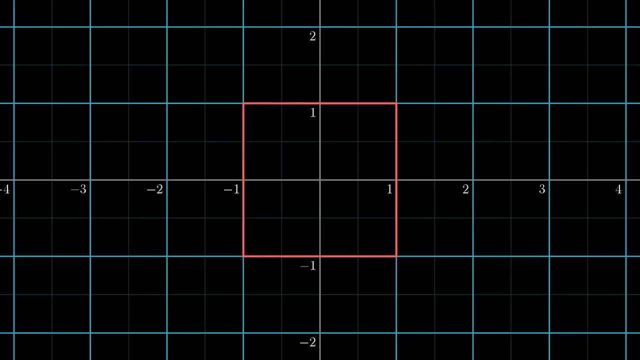 of something that seems reasonable and even dull in 2 and 3 dimensions, But which is not, Which is totally out of whack in higher dimensions. To start, take a 2x2 box, centered at the origin: Its corners are on the vertices and 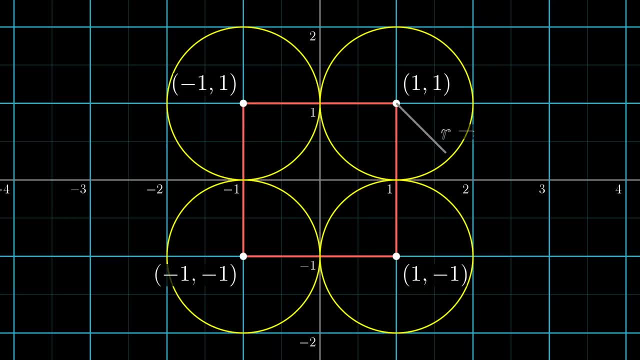 Draw four circles, each with radius 1, centered at these four vertices, So each one is tangent to two of its neighbors. Now I want you to think of the circle centered at the origin, which is just large enough to be touching those corner circles. 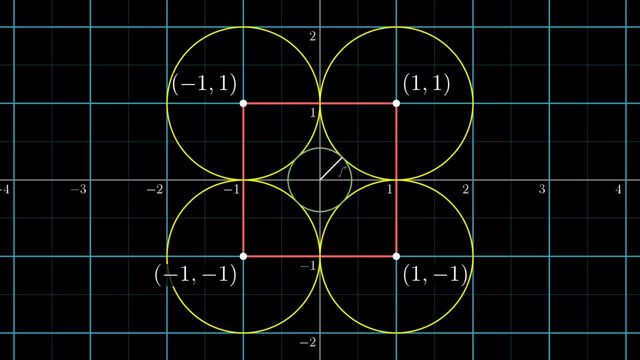 What we want to do for this setup and for its analogies in higher dimensions is find the radius of that inner circle Here in two dimensions. we can use the Pythagorean theorem to see that the distance from the origin to the corner of the box is the square root of 2,, which is around 1.414.. 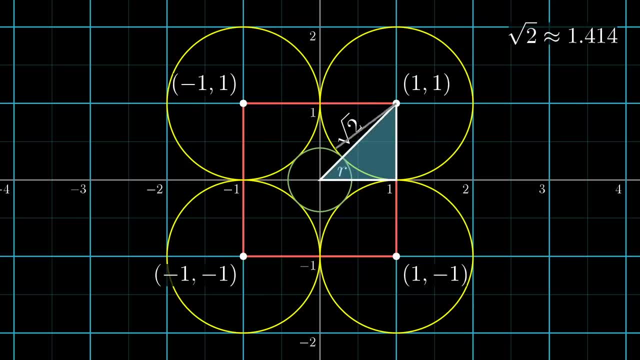 Then you can subtract off this portion here the radius of the corner circle, which by definition is 1.. Therefore the radius of that inner circle is square root of 2 minus 1, or about .414.. 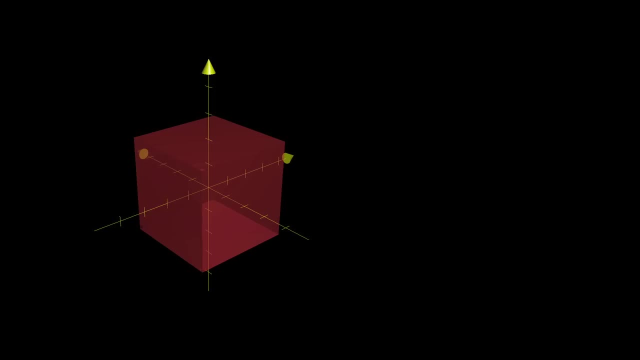 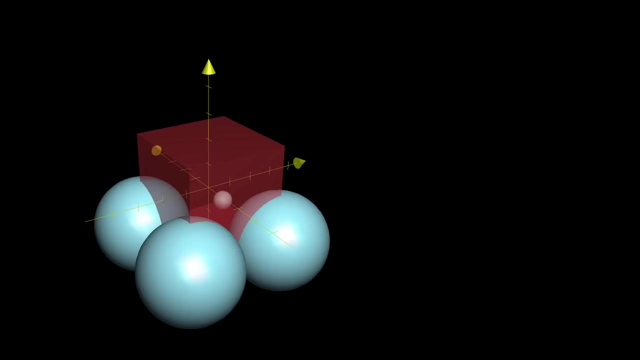 No surprises here. That seems quite reasonable. Now do something analogous in three dimensions. Draw a 2x2x2 cube whose corners have vertices, and on and on, And then we're going to take 8 different spheres, each of which has a radius 1, and. 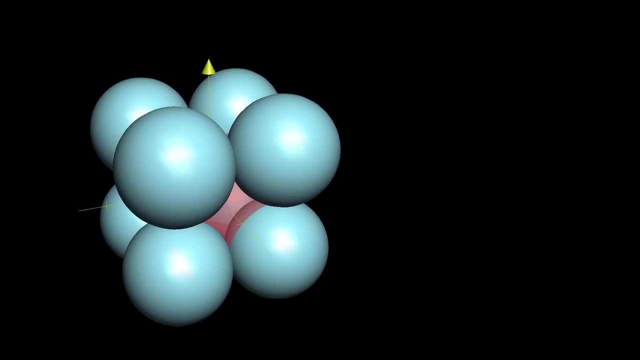 center them on those vertices so that each one is tangent to 3 of its neighbors. And then we're going to set 8 different spheres, each of which has a radius 1, and center them on these vertices so that each one is tangent to three of its neighbors. 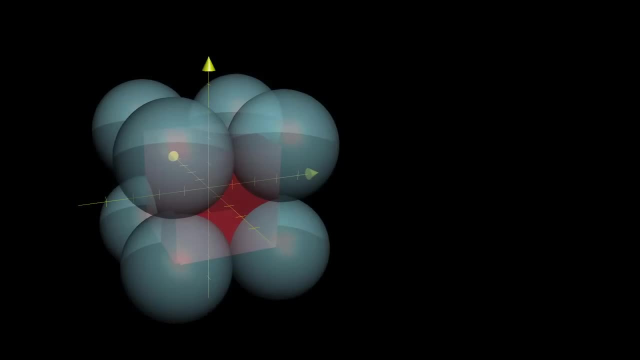 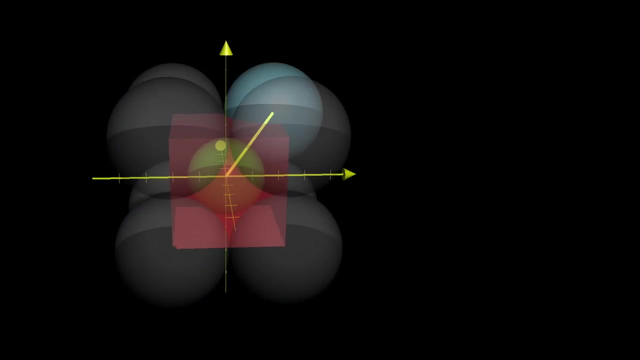 neighbors. Now again, think about the sphere centered at the origin, which is just large enough to be barely touching those 8 corner spheres. As before, we can start by thinking about the distance from the origin to the corner of the box, say the corner at. 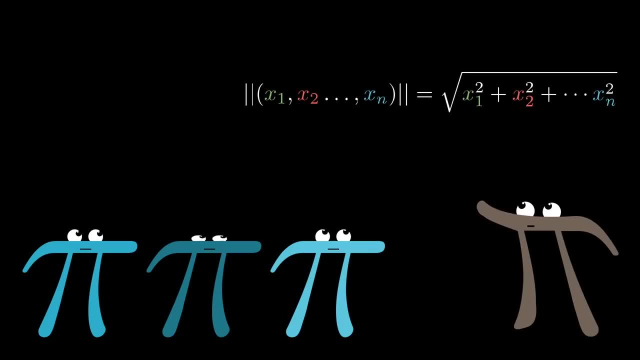 By the way, I guess I still haven't yet explicitly said that the way distances work in higher dimensions is always to add up the squares of the components in each direction and take the square root. If you've never seen why this follows from the Pythagorean theorem, just in the two-dimensional 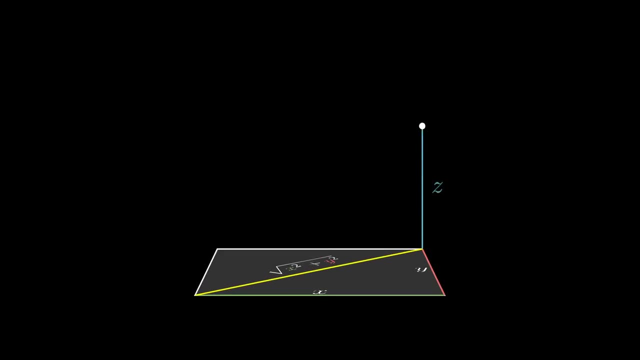 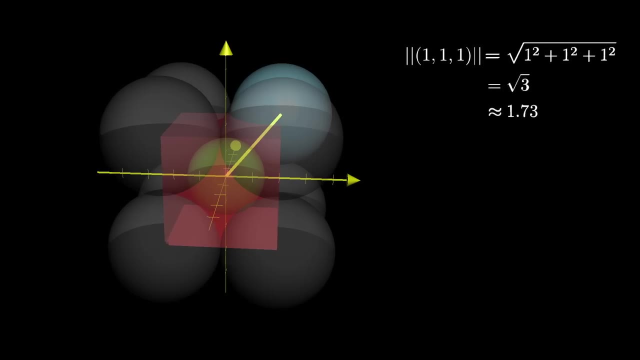 case. it's actually a really fun puzzle to think about, and I've left the relevant image up on the screen for any of you who want to pause and ponder on it. Anyway, in our case, the distance between the origin and the corner is the square. 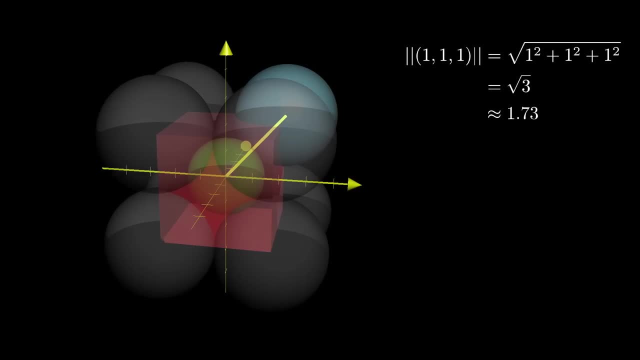 root of or square root of 3, which is about 1.73.. So the radius of that inner sphere is going to be this quantity minus the radius of a corner sphere, Which by definition is 1.. And again 0.73 seems like a reasonable radius for that inner sphere. 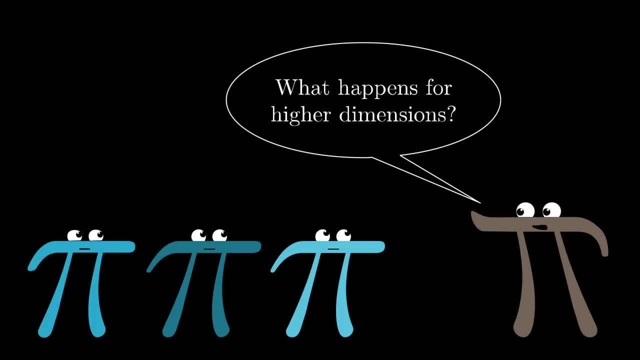 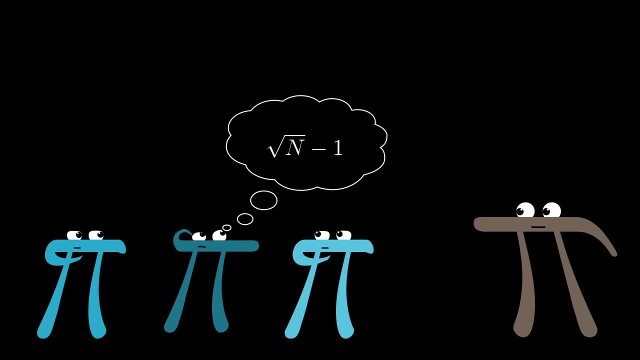 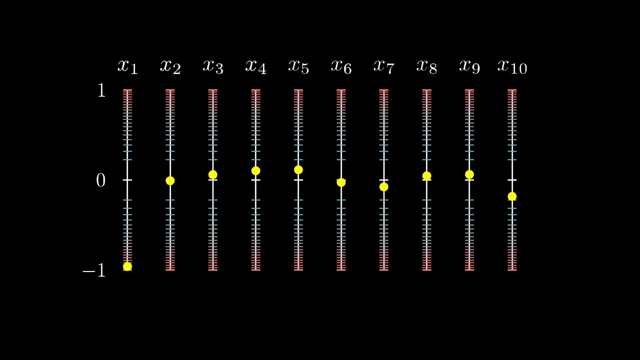 But what happens to that inner radius as you increase dimensions? Obviously, the reason I bring this up is that something surprising will happen and some of you might see where this is going, But I actually don't want it to feel like a surprise. As fun as it is to wow people with counter-intuitive facts and math, the goal here is genuine understanding. 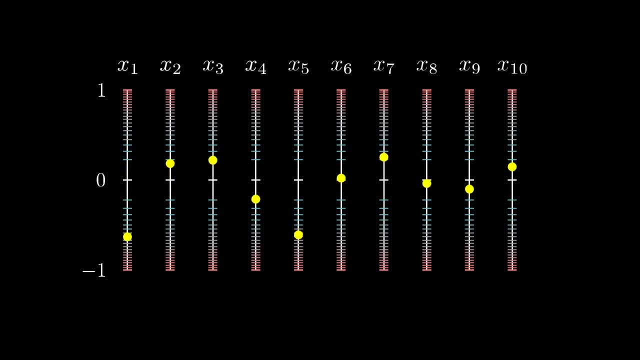 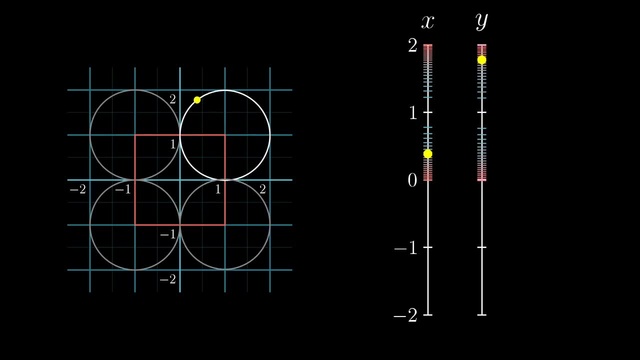 not shock. For higher dimensions. we'll be using sliders to get a gut feel for what's going on, But since it's kind of a different way of viewing things, it helps to get a running start by looking back at how to analyze the 2- and 3-dimensional cases in the context. 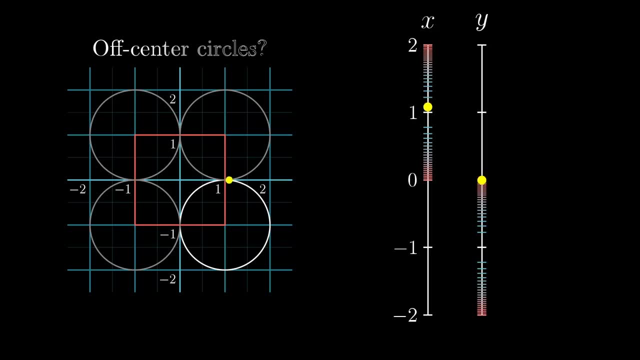 of sliders. First things first. how do you think about a circle centered at a corner like 1, negative 1?? Well, previously, for a circle centered at the origin, the amount of real estate belonging to both x and y was dependent on their distance from the number 0. 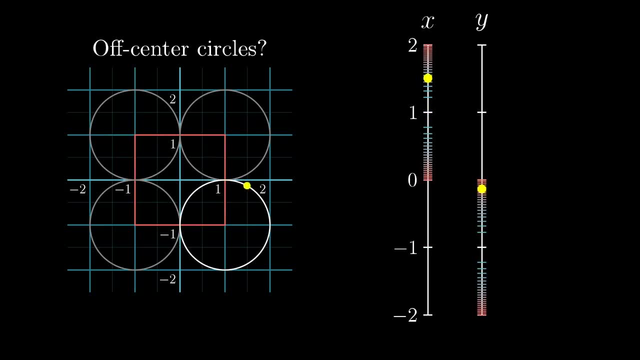 And it's the same basic idea here as you move around the center. it's just that the real estate might be dependent on the distance between each coordinate and some other number. So for this circle centered at the amount of real estate belonging to x is the. 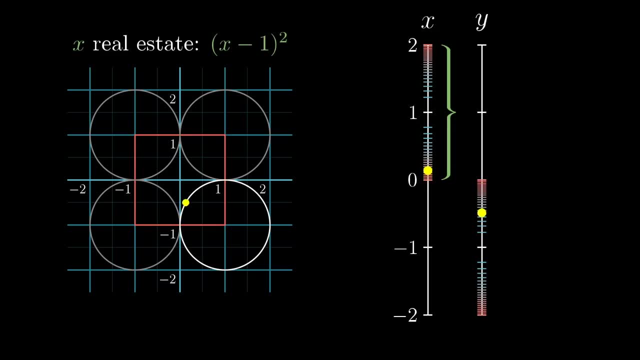 square of its distance from 1.. Likewise, the real estate belonging to y is the square of its distance from negative 1.. Other than that, the look and feel with this piston dance trade-off is completely the same. For simplicity, we'll only focus on one of these circles, the one centered at 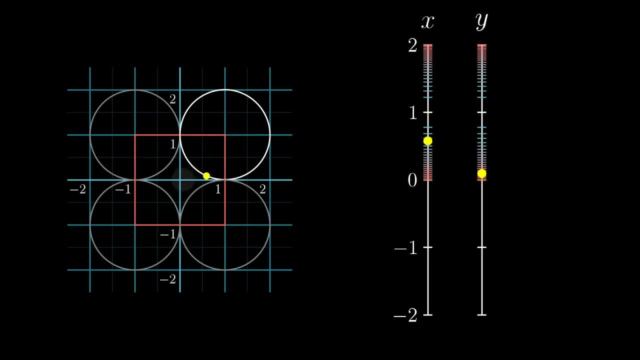 Now ask yourself: what does it mean to find a circle centered at the origin large enough to be tangent to this guy, when we're thinking just in terms of sliders? Well, notice how this point of tangency happens when the x and y coordinates are both the 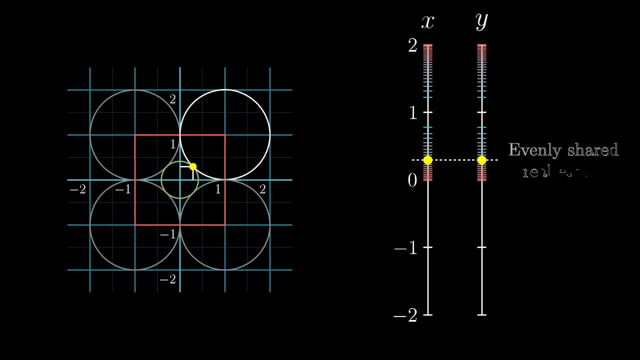 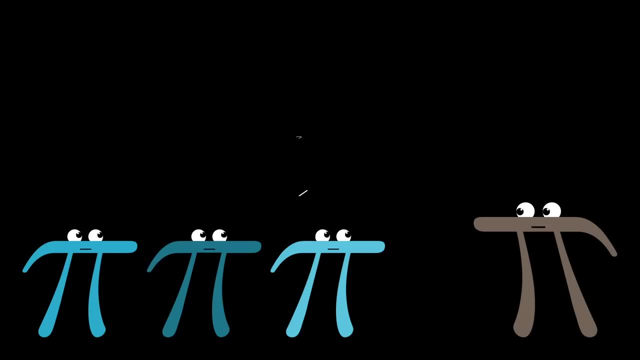 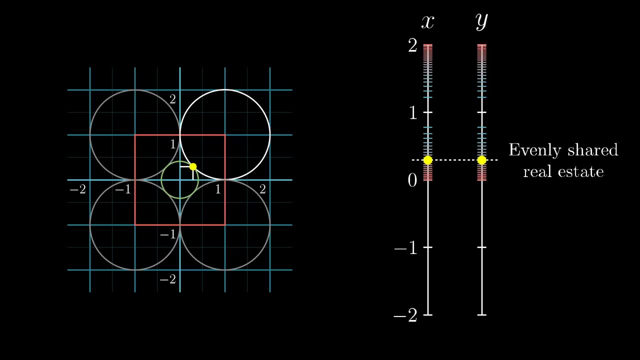 same Or phrased differently. at the point of this corner circle, closest to the origin, the real estate is shared evenly. This will be important for later, so let's dig in and think about why it's true. Imagine perturbing that point slightly, maybe moving x a little closer to 0, which means 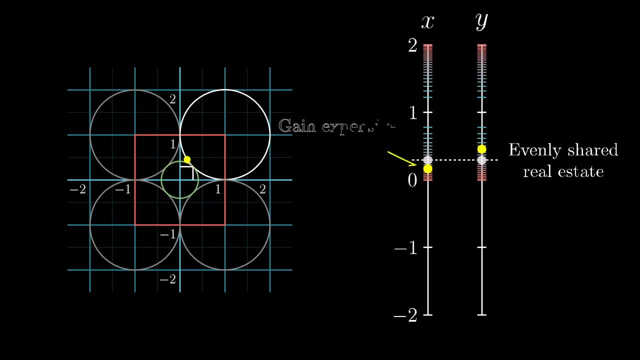 y would have to move a little away from 0.. The change in x would have to be a little smaller than the change in y, since the real estate it gains by moving farther away from 1 is more expensive than the real estate y loses by getting closer to 1.. 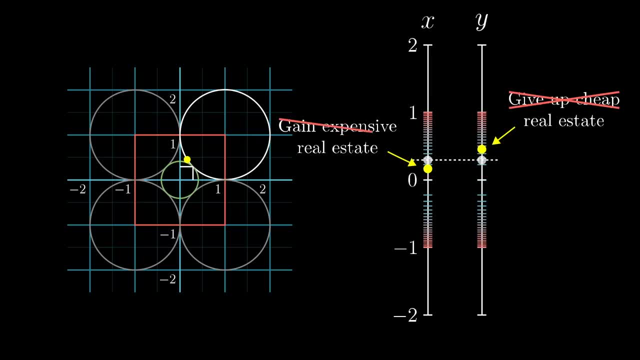 But from the perspective of the origin point it's not the same. The change in x would have to be a little smaller than the change in y. since the real estate is measured with respect to 0, and the result is reversed, The resulting change to x squared is smaller than the resulting change to y squared, since 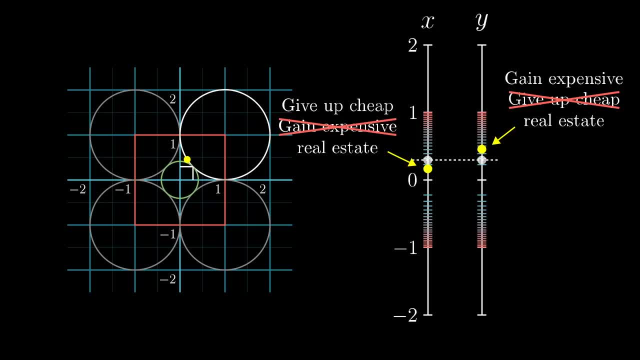 when real estate is measured with respect to 0, that move of y towards 1 is the more expensive one. What this means is that any slight perturbation away from this point where real estate is shared evenly, results in an increasing distance from the origin. 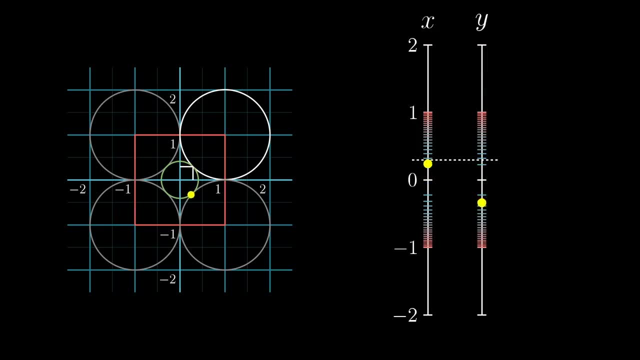 The reason we care is that this point is tangent to the origin point and we don't want to lose the point. It's tangent to the inner circle, so we can also think about it as being a point of the inner circle, And this will be very useful for higher dimensions. it gives us a reference point to understanding. 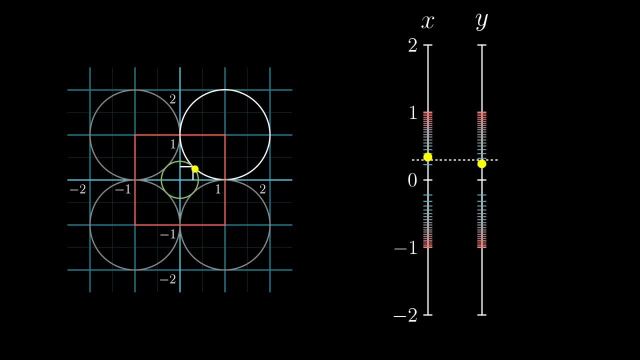 the radius of that inner circle. Specifically, you can ask how much real estate is shared between x and y at this point, when real estate measurements are done with respect to the origin 0, 0.. For example, down here, in two dimensions, both x and y dip below 0.5 in this configuration. 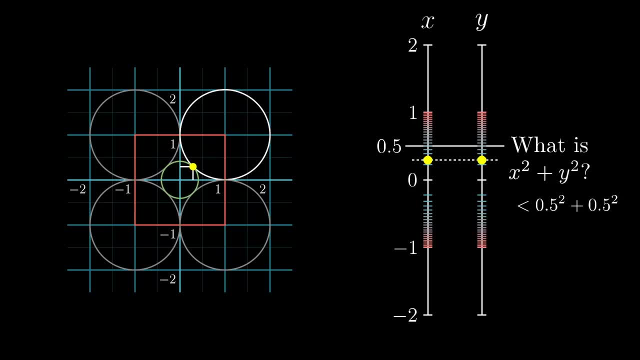 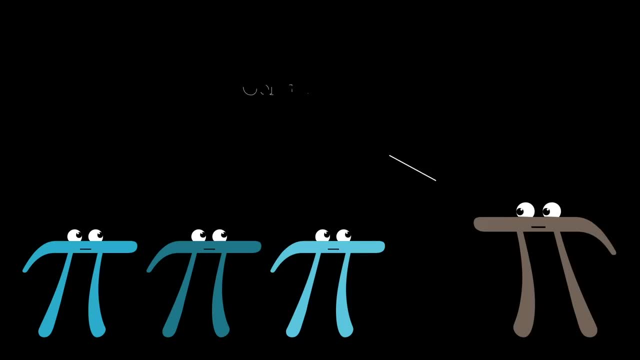 This is because x and y dip below 0.5.. So the total value x squared plus y squared is less than 0.5 squared plus 0.5 squared. Comparing to this halfway point is really going to come in handy for wrapping our mind. 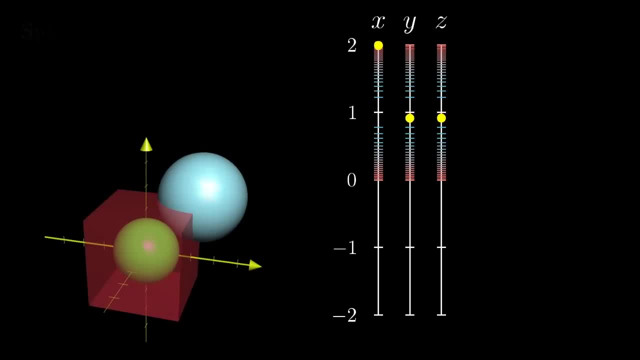 around what happens in higher dimensions. Taking things one step at a time, let's bump it up to three dimensions. Consider the corner sphere with radius 1, centered at The point on that sphere closest to the origin, corresponds to the configuration of the inner circle. 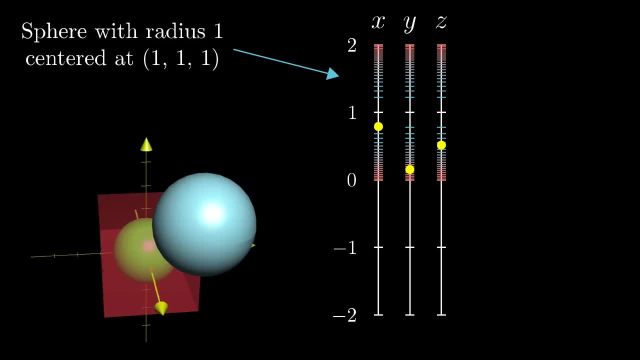 The point on that sphere that's closest to the origin corresponds to the configuration of the inner circle. The point on that sphere is the position of sliders, where x, y and z are all reaching down toward 0 and equal to each other. 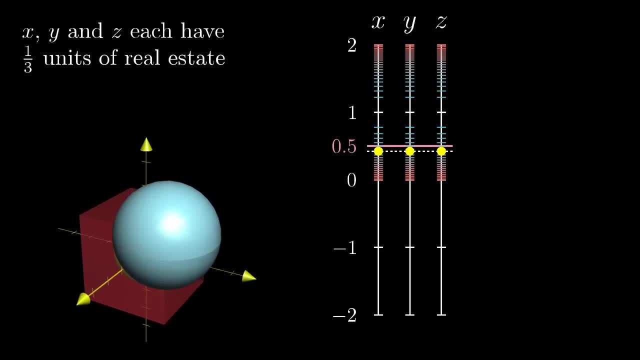 Again, they all have to go a little beyond that halfway point because the position 0.5 only accounts for 0.5 squared or 0.25 units of real estate. So with all three coordinates getting a third of a unit of real estate they need to be. 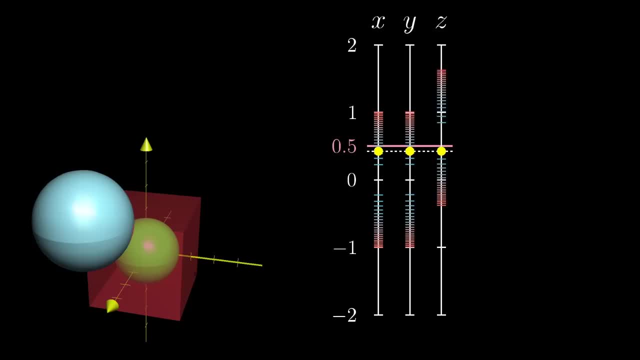 farther out. And again, since this is a point where the corner sphere is tangent to the inner sphere, it's also a point where the corner sphere is tangent to the inner sphere. So, with reference to the origin, 0, 0, 0, think about the amount of real estate shared. 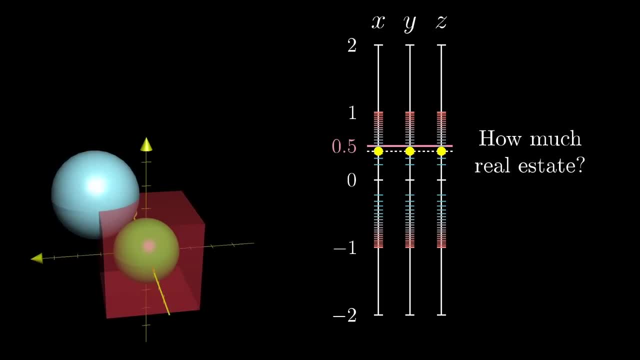 between x, y and z. in this position, corresponding to the tangent point, It's definitely less than 0.75, since all three of these are smaller than 0.5.. So each one has less than 0.25 units of real estate. 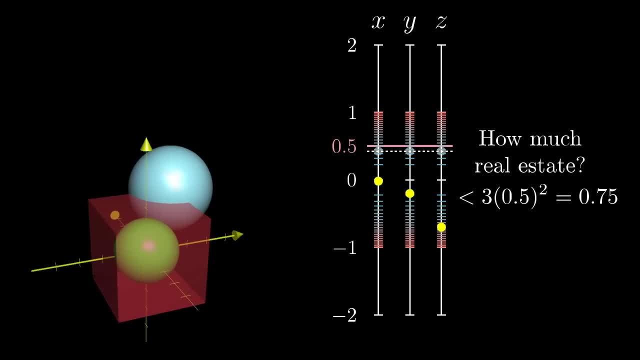 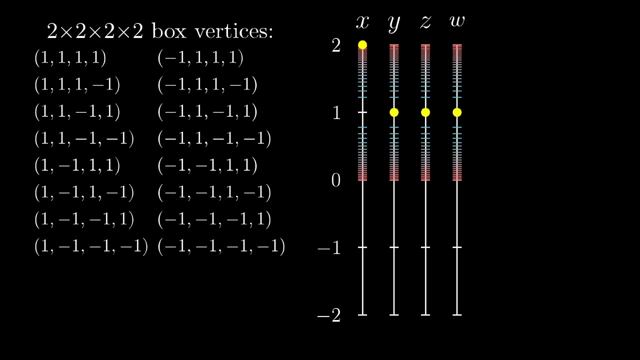 And again we sit back and feel comfortable with this result. right, the inner sphere is smaller than the corner spheres, But things get interesting when we move up into four dimensions. Our 2x2x2x2 box is going to have 16 vertices at, and so on with all possible binary. 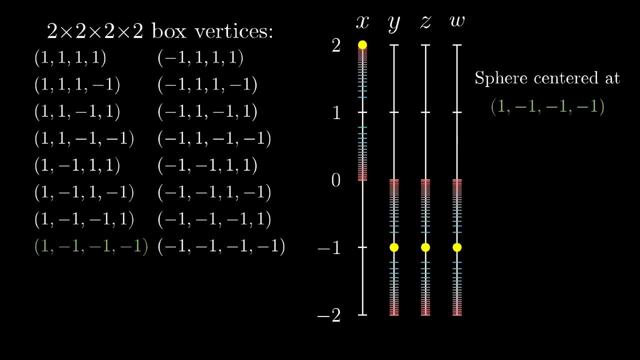 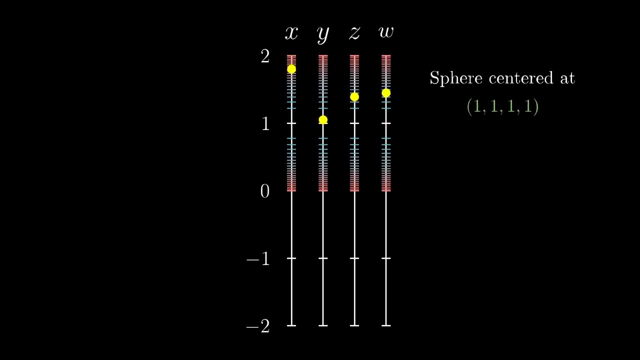 combinations of 1, and What this means is that there are 16 unit spheres centered at these corners, each one tangent to four of its neighbors. As before, we'll just be focusing on one of them. the one centered at The point of the sphere closest to the origin corresponds to the configuration of sliders. 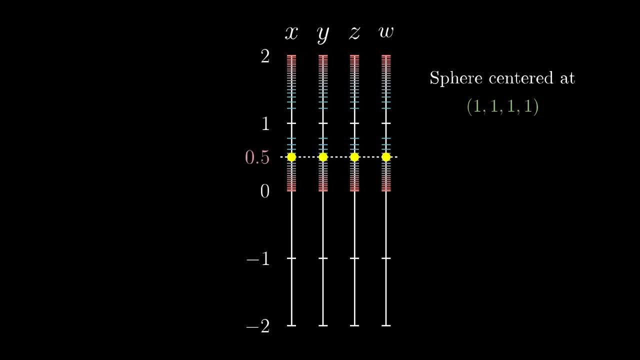 where all four coordinates reach exactly halfway between 1 and 0. And that's because, when one of the coordinates is 0.5 units away from 1, it has 0.25 units of real estate with respect to the point 1.. 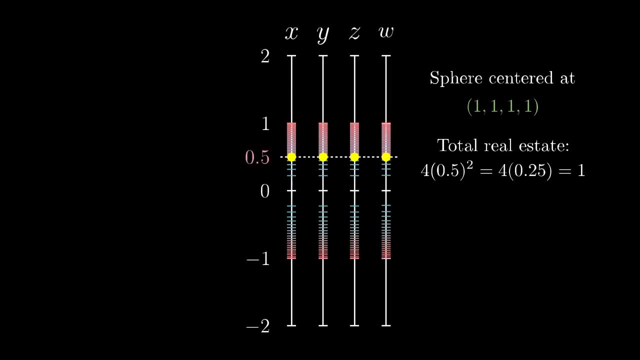 We do the same trick as before: thinking of this now as a point of the inner sphere and measuring things with respect to the origin, But you can already see what's cool about four dimensions As you switch to thinking of real estate with respect to. it's still the case that 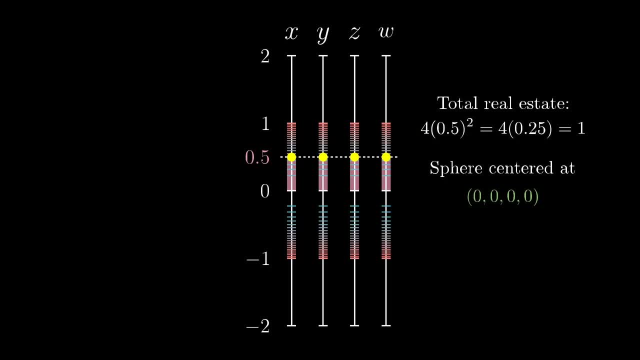 each of these four coordinates has 0.25 units of real estate, making for a total of one shared between the four coordinates. In other words, that inner sphere is precisely the same size as the corner spheres. This matches with what you see numerically, by the way. 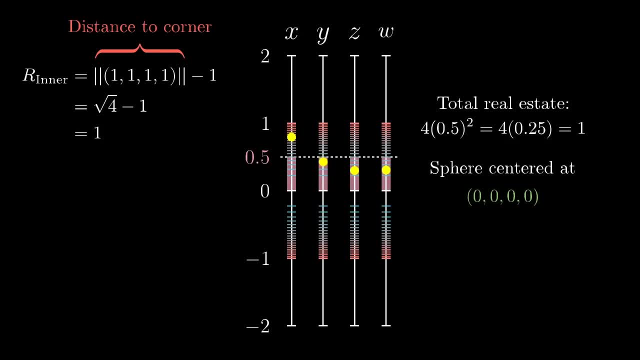 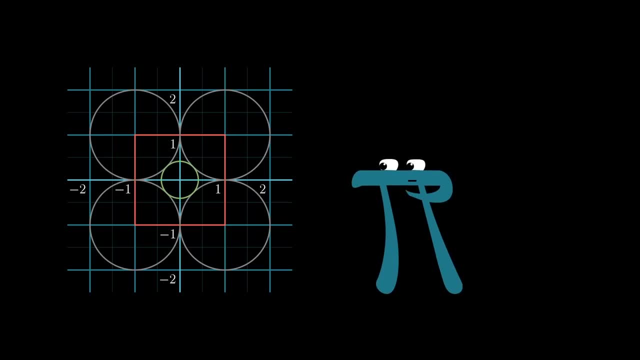 the 2x2x2x2 box And when you're stuck thinking in the 2- or 3-dimensional cases, this fact that the inner sphere has radius 1, the same size as the corner spheres, and that it touches the 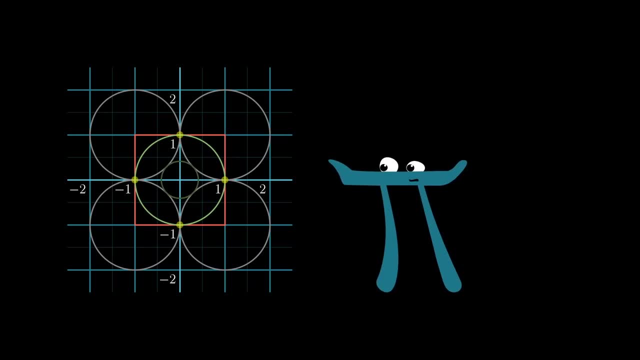 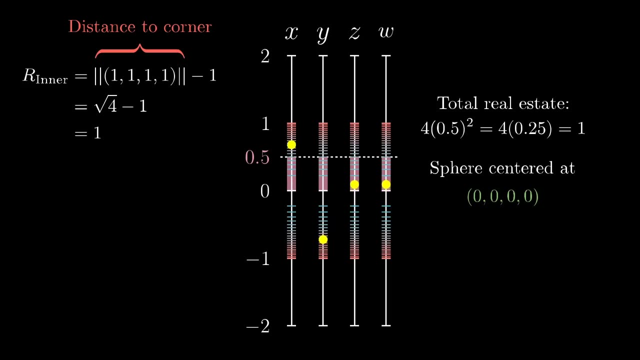 box. well, it just seems too big, But it's important to realize this is fundamentally a 4-dimensional phenomenon and you just can't cram it down into smaller dimensions, But things get weirder. let's knock it up to 5 dimensions. 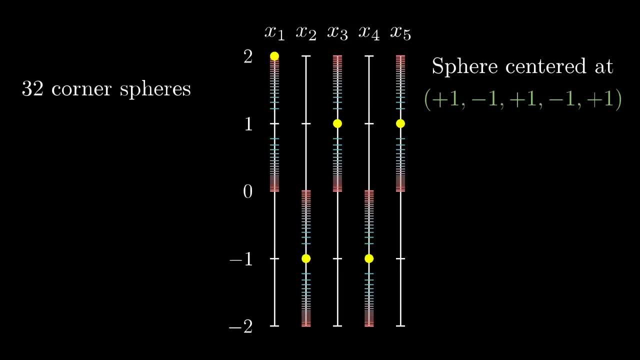 In this case we have quite a few corner spheres, 32 in total, But again, for simplicity, we'll only be thinking about the ones centered at. Think about the point of this sphere closest to the origin, where all 5 coordinates are. 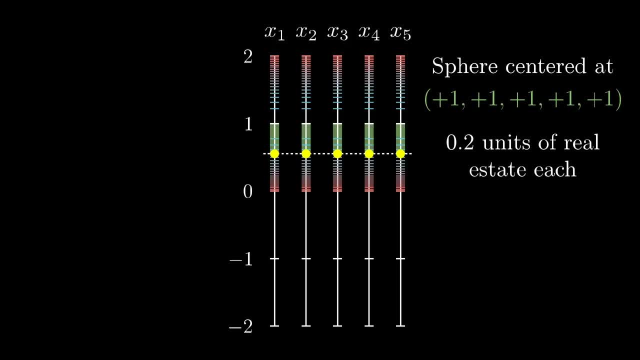 equally splitting the 1 unit of shared real estate. This time each coordinate is a little higher than 0.5.. If they reach down to 0.5, each one would have 0.25 units of real estate, giving a total. 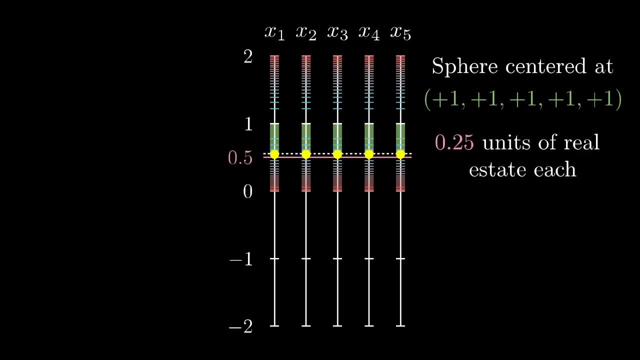 of 1.25,, which is too much. But the tables are turned when you view this as a point on the inner sphere, because, with respect to the origin, this configuration has much more than 1 unit of real estate. Not only is every coordinate more than 0.5 units away from 0, but the larger number of 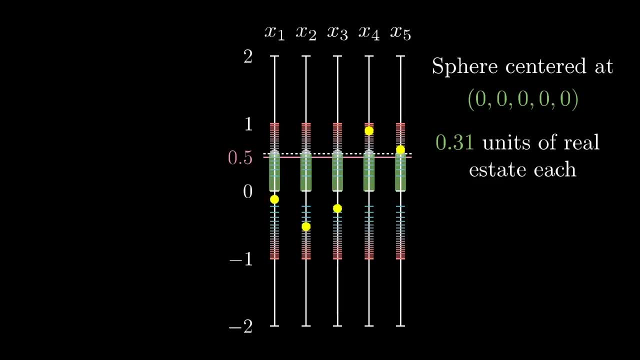 dimensions means that there's more total real estate. when you add it all up Specifically, you can compute that the radius of that inner sphere is about 1.24.. The intuitive theory is that the radius of that inner sphere is about 1.24.. 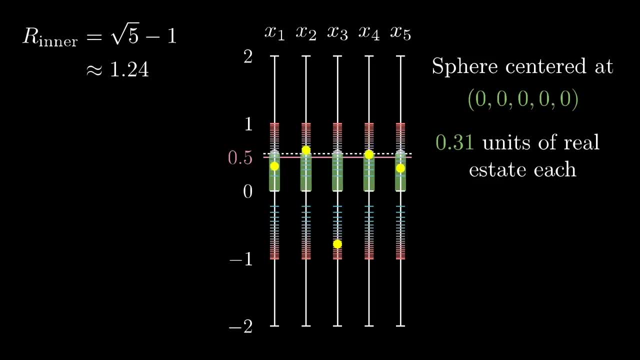 The intuitive theory is that the radius of that inner sphere is about 1.24.. What's interesting is that you can actually get the feeling the sliders can actually roam over more territory than just a single unit of real estate can. One fun way to see what this means is to adjust everything so that all real estate goes to. 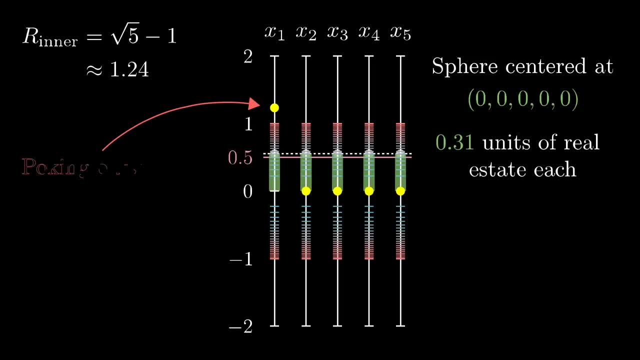 just one coordinate, Because this coordinate can reach beyond one. what you are seeing is that this 5-dimensional sphere actually pokes in in皆さん, and today's very small space is happening just outside the box. But to really get a feel for how strange things become, I can just tell you now that we've 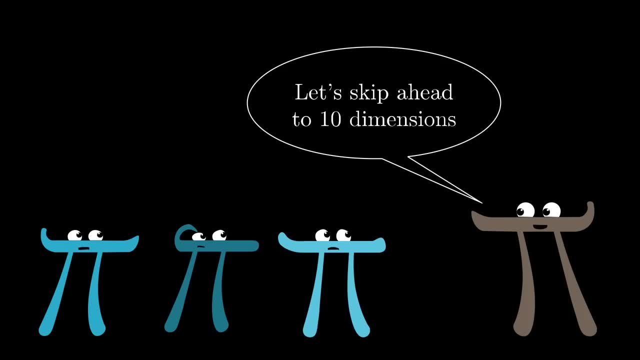 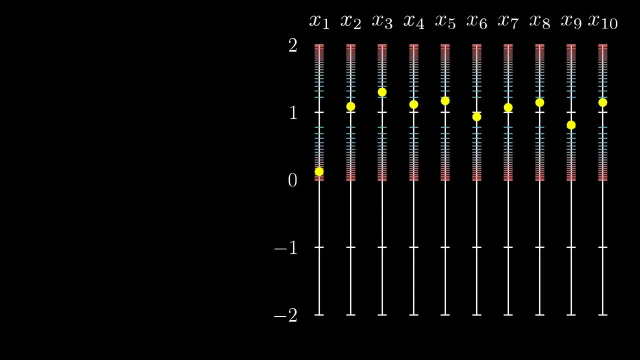 only had one perfect slide up into 10 dimensions. Remember all this means is that points have 10 coordinates. For a sphere with radius 1, a single unit of real estate must be shared among all 10 of those coordinates. As always, the point of this corner sphere closest to the origin is the one where all 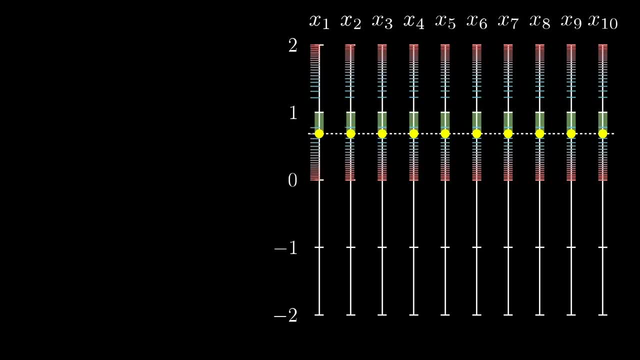 10 coordinates split the real estate evenly, And here you can really see just how far away this feels from the origin. Or, phrased differently, that inner sphere is allowed to have a very large amount of real estate. In fact, you can compute that the radius of the inner sphere is about 2.16.. 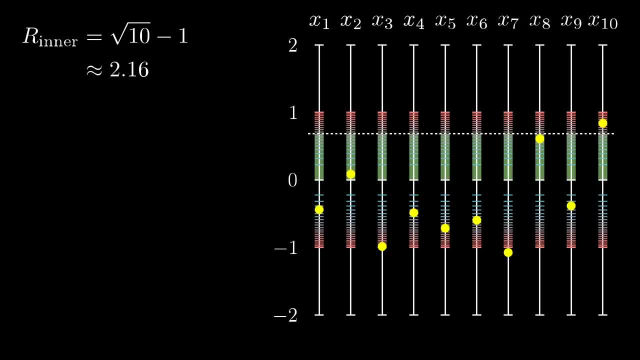 And viewed from this perspective, where you have 10 full dimensions to share that real estate, doesn't it actually feel somewhat reasonable that the inner sphere should have a radius more than twice as big as all those corner spheres? To get a sense for just how big this? 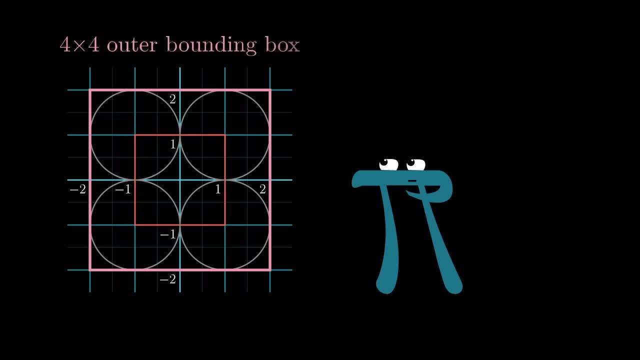 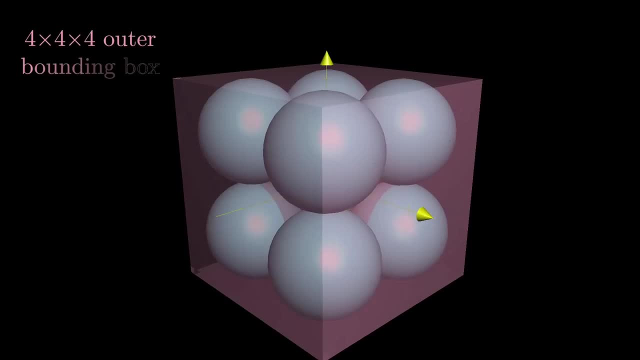 inner sphere is. look back in two dimensions and imagine a 4x4 box bounding all four sources of the inner sphere to the outer sphere of the inner sphere. And here you can see that the outer sphere is a 4x4 box bounding all the corner spheres from the outside. 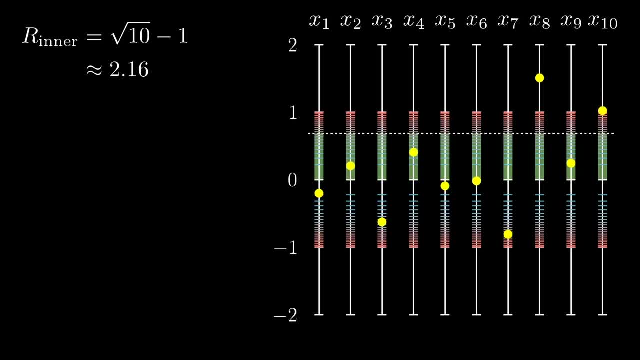 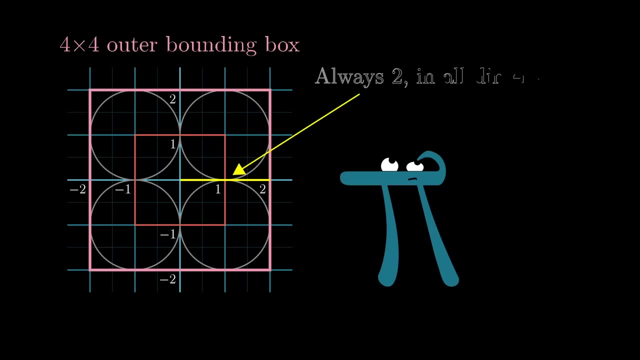 Way up here in 10 dimensions. that- quote unquote- inner sphere is actually large enough to poke outside of that outer bounding box, since it has a diameter bigger than 4.. I know that seems crazy, but you have to realize that the face of the box is always 2 units of real estate. 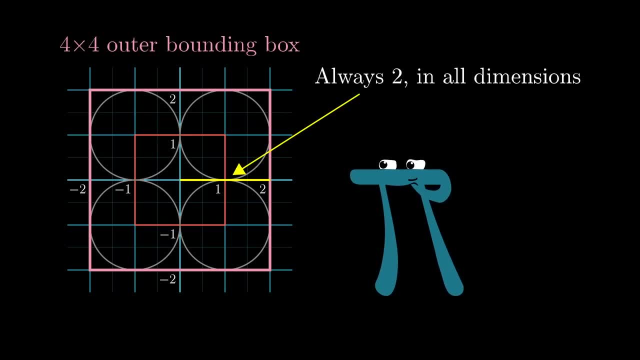 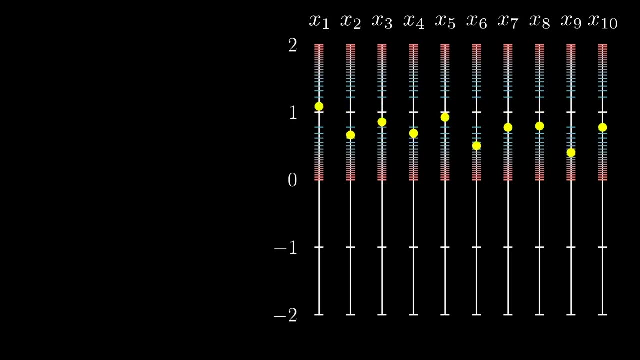 The inner sphere is only 2 units away from the origin, no matter how high the dimension is, And fundamentally it's because it only involves moving along a single axis, But the point 111111111,, which determines the inner sphere's radius, is actually really far. 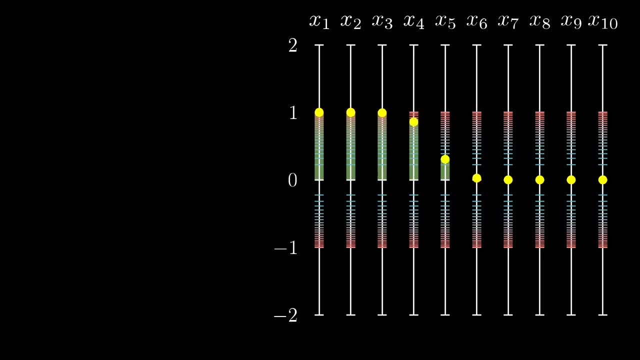 away from the center all the way up here in 10 dimensions, And it's because all 10 of those dimensions add a full unit of real estate for that point. And of course, as you keep upping the dimensions, that inner sphere just keeps growing. 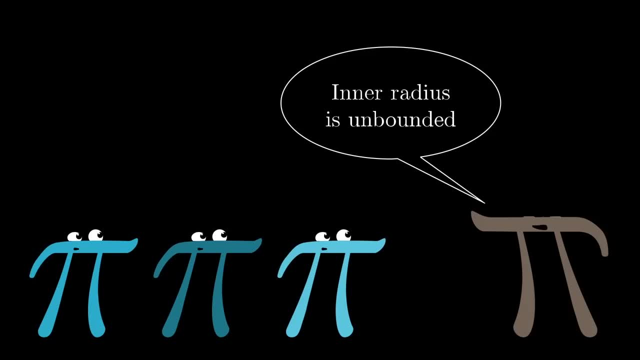 And of course, as you keep upping the dimensions, that inner sphere just keeps growing. And of course, as you keep upping the dimensions, that inner sphere just keeps growing, Not only is it poking outside of these boxes, but the proportion of the inner sphere. 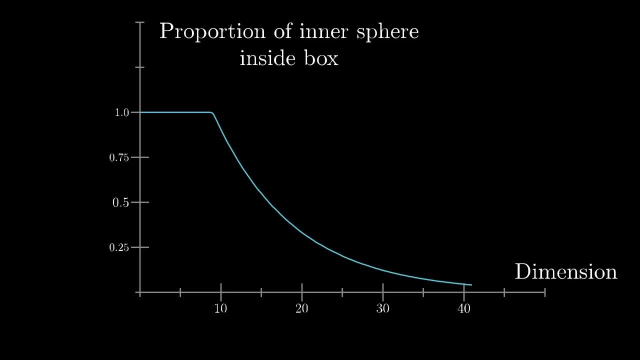 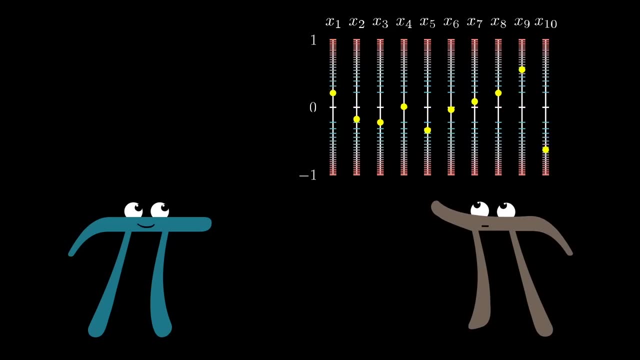 lying inside the box decreases exponentially towards zero as the dimension keeps increasing. So taking a step back. one of the things I like about using this slider method for teaching is that when I shared it with a few friends, the way they started to talk about higher dimensions. 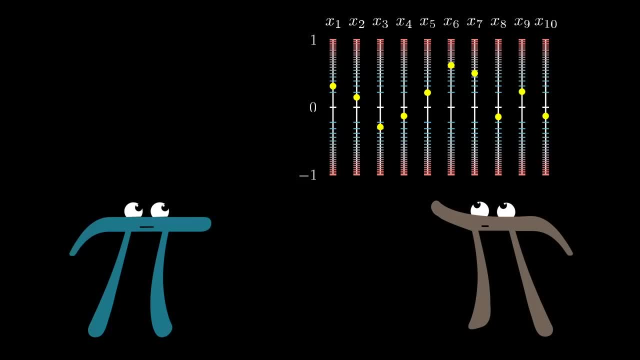 became a little less metaphysical and started to sound more like how you would hear a mathematician talk about the topic. a little less metaphysical and started to sound more like how you would hear a mathematician talk about the topic- the topic- Rather than skeptically asking whether or not 10-dimensional space is a real thing. 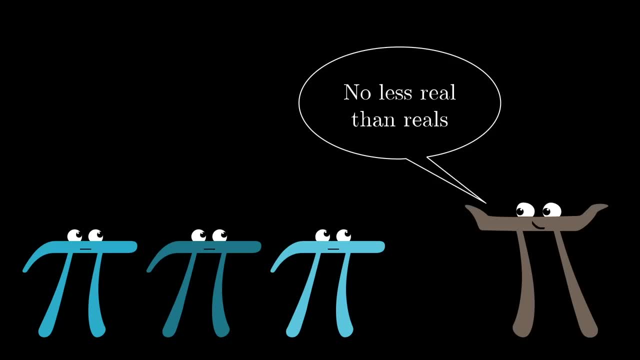 recognizing that it's exactly as real as numbers are. people would actually probe at what other properties high-dimensional spheres have and what other shapes feel like in terms of sliders. This box situation is just one in a number of things that feel very crazy about higher. 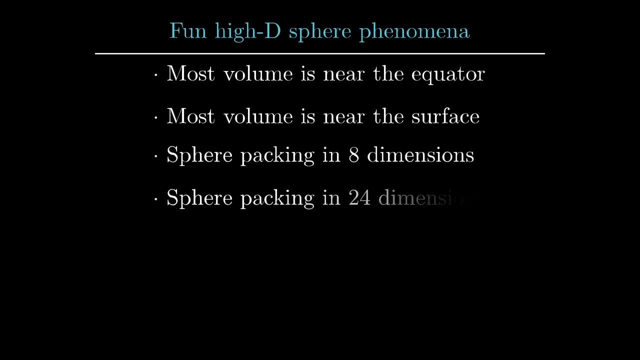 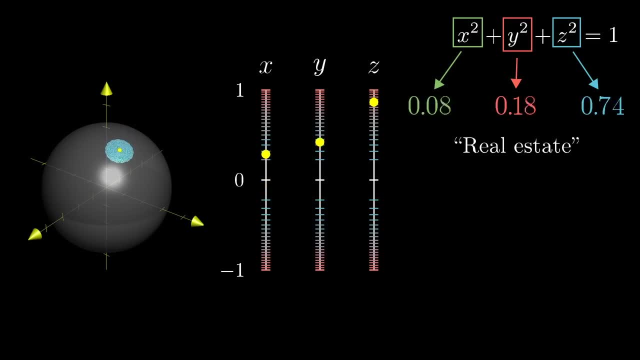 dimensional spheres and it's really fun to think about these others in the context of sliders and real estate. It's obviously limited. I mean, you're a bug on the surface of these objects, only getting a feel for one point at a time and for the rules of movement. 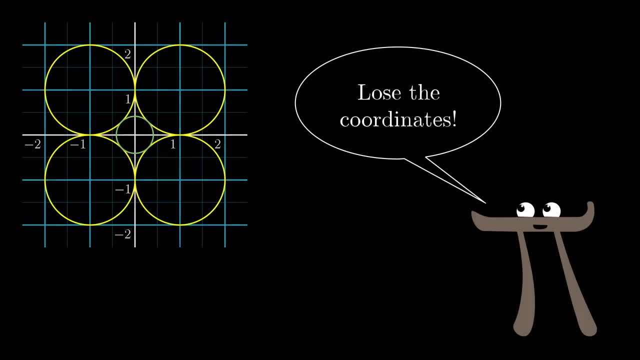 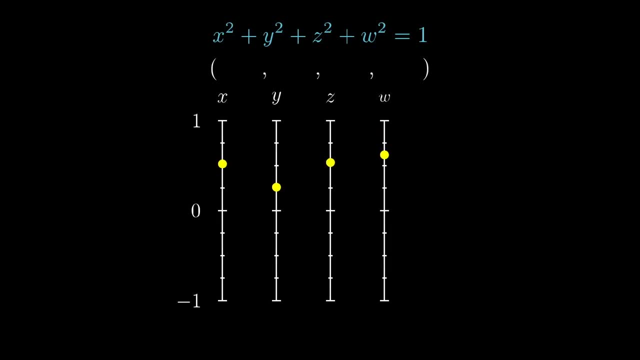 Also, geometry can be quite nice when it's coordinate free- and this is the opposite of that- but it does give a foothold into thinking about high dimensional shapes a little more concretely. Now you could say that viewing things with sliders is no different from thinking about. things purely analytically. I mean, it's honestly a little bit more complicated to think about high-dimensional shapes than you'd think of sliders. I mean, it's honestly a little bit more complicated to think about high-dimensional shapes than you'd think of sliders. 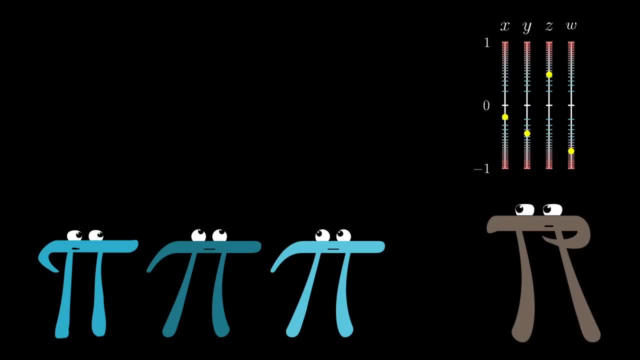 more than representing each coordinate literally. it's kind of the most obvious thing you might do, But this small move makes it much more possible to play with the thought of a high dimensional point And even little things like thinking about the squares of coordinates as real estate. 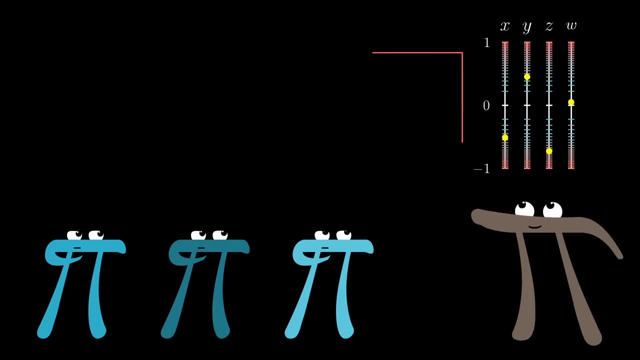 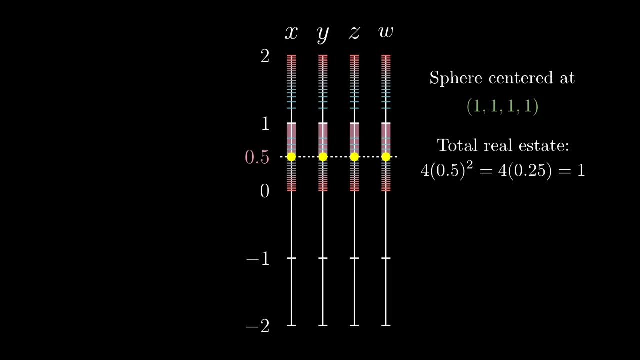 can shed light on some seemingly strange aspects of high dimensions, like just how far away the corner of a box is from its center. If anything, the fact that it's such a direct representation of a purely analytic description is exactly what makes it such a faithful reflection of what genuinely doing math in higher dimensions entails. 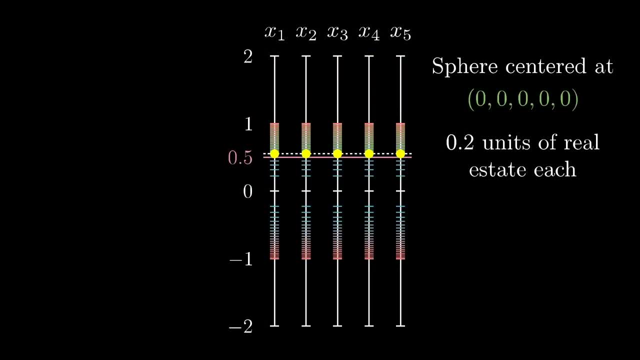 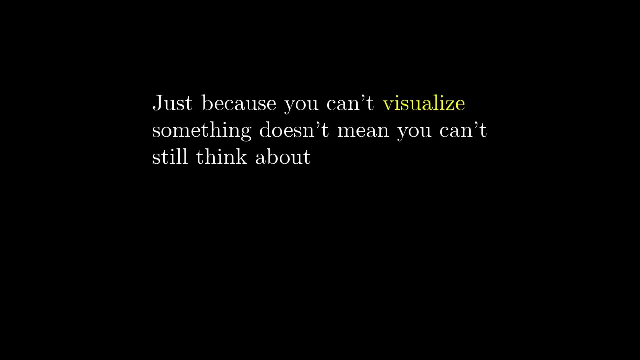 We're still flying in the clouds, trusting the instruments of analytic reasoning, but this is a redesign of those instruments, one which better takes advantage of the fact that such a large portion of our brains goes towards image processing. I mean, just because you can't visualize something doesn't mean you can't still think about it visually.